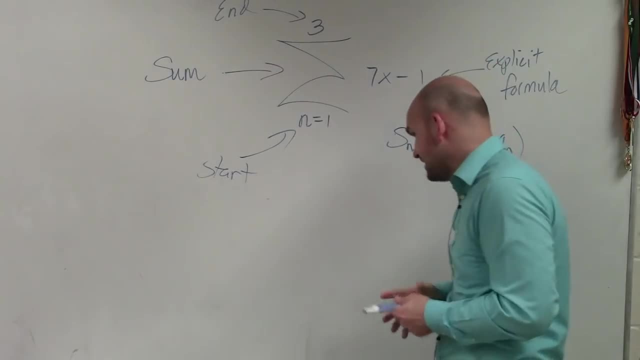 This is what sigma represents. And here is your end. All right, now I'll explain my way through it once I divide. Because when you guys get a test, you're just going to look like this And it's going to say: hey, question number one. And it's going to look like that, It's going to 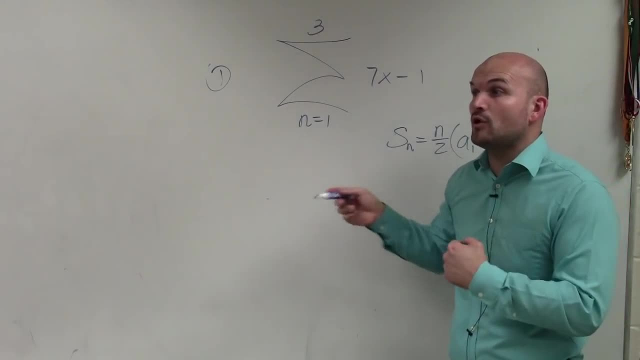 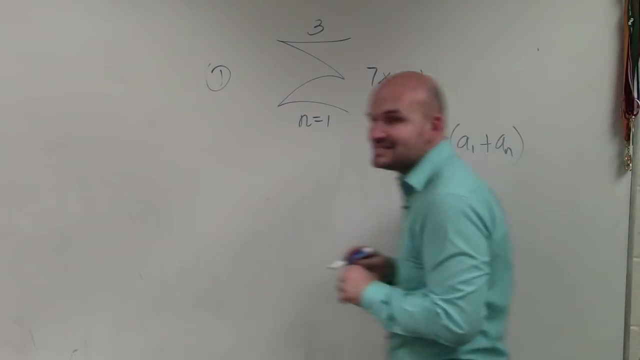 say what's the answer, And so what you're going to have to know is: oh, they're asking me for the sum, Not right now. I'm explaining something that we really need to make sure we know where it is. So we have s of n equals n divided by 2 times a sub 1 plus n, a sub n. Do we know what the 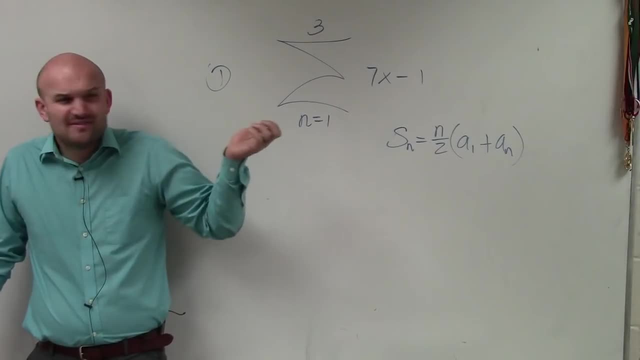 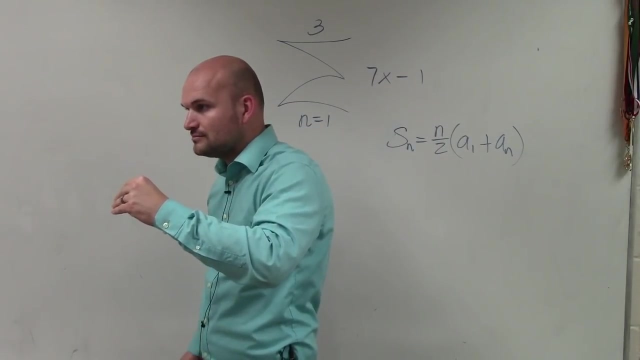 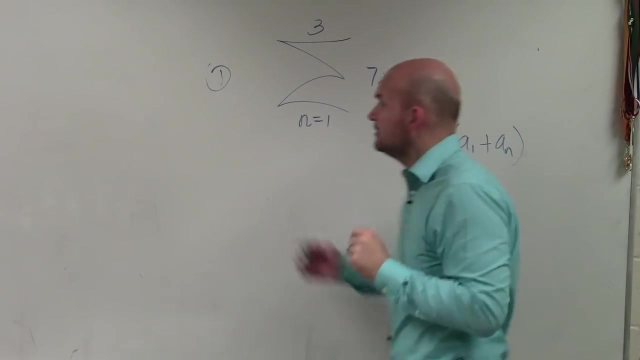 first number is of our sequence. Do we even have a sequence? Well, we only have a formula, this explicit formula, And, if you guys remember, 3, which represents the end. Okay, so if you guys remember how we wrote explicit formulas, 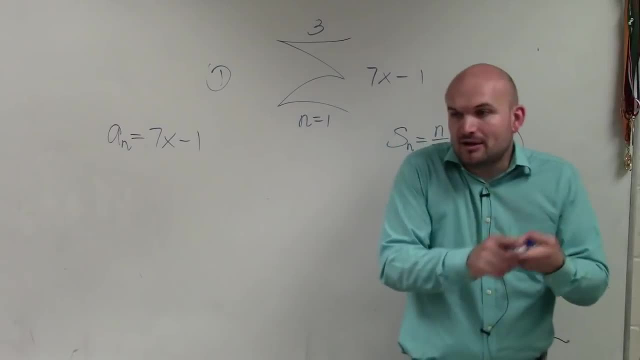 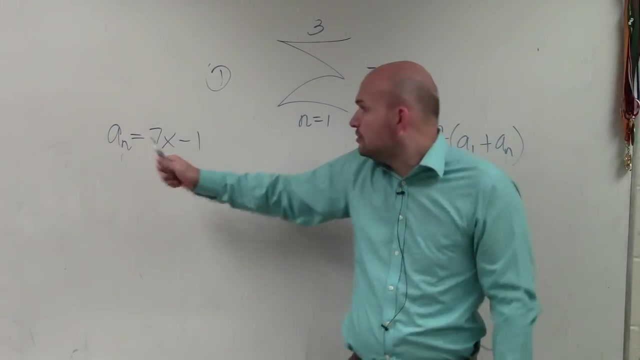 We wrote explicit formulas as like a sub n. right, It could have been arithmetic, It could have been geometric, It doesn't really matter. This is like. your explicit formula can also be written as this: Oops, where n? Where is this x I'm using? sorry? Sorry, there's no x We're using. 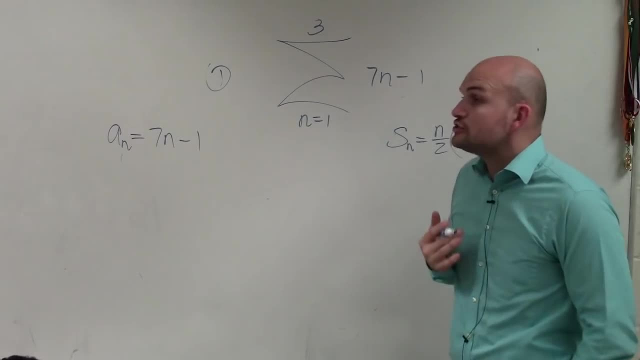 n's here. n represents the number of the sequence. Sorry, I got mistaken. So can we figure out what the first term is? though, once we know what the formula is, Yeah, you just plug in the first number, right. 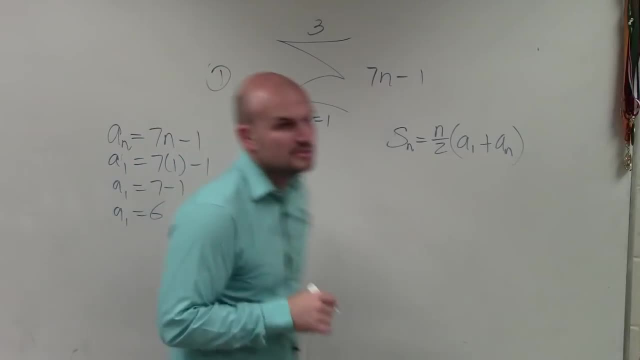 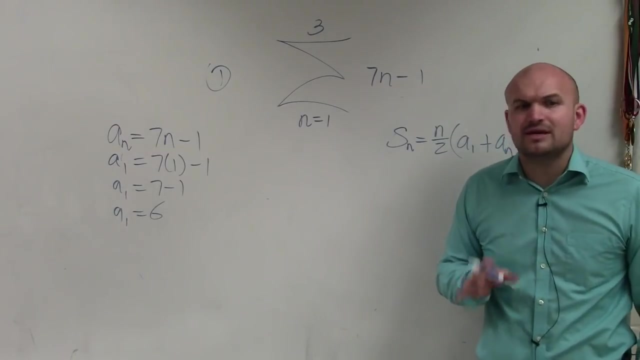 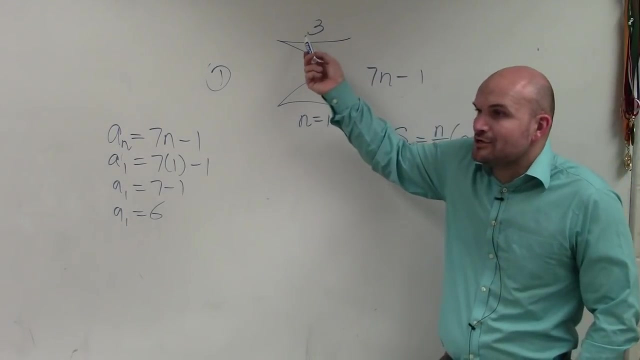 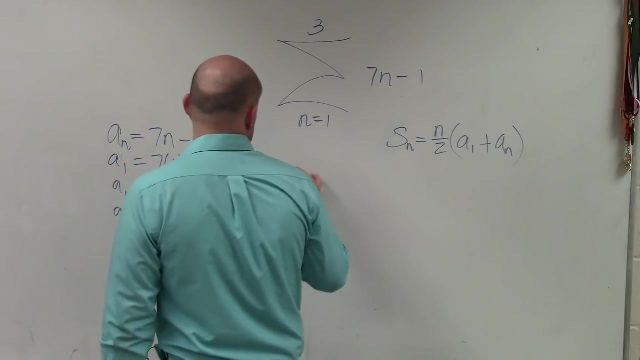 Does everybody see that? Does everybody see that? Okay, Now the next thing. Mario, I'm really having a hard time. I really am. The next thing is: what is our last term? The last term is well, what is the last term? it ends with 3.. Can we find out what a sub 3 is? Okay, Yep, So now you just 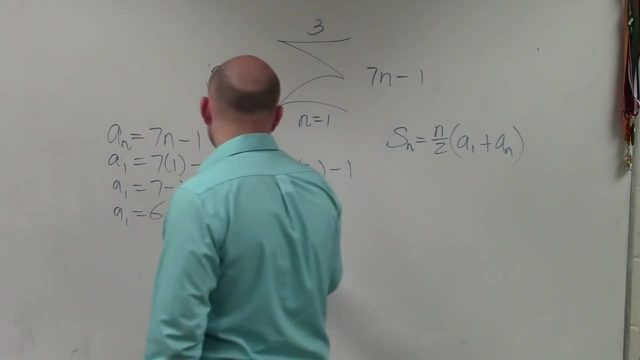 plug 3 in for n 7 times 3 is 20.. Okay, So now you just plug 3 in for n 7 times 3 is 20.. So now you just plug 3 in for n 7 times 3 is 21.. Minus 1 is 20.. So, Kelsey, you're not giving it a shot. 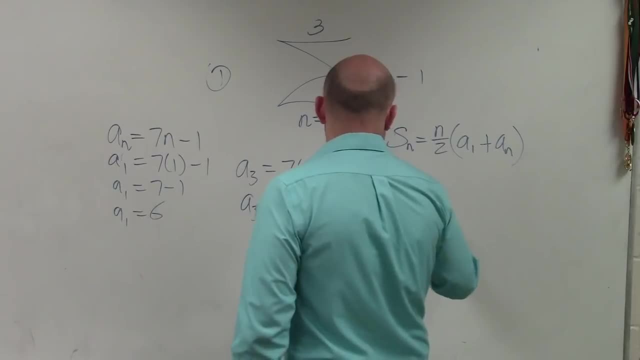 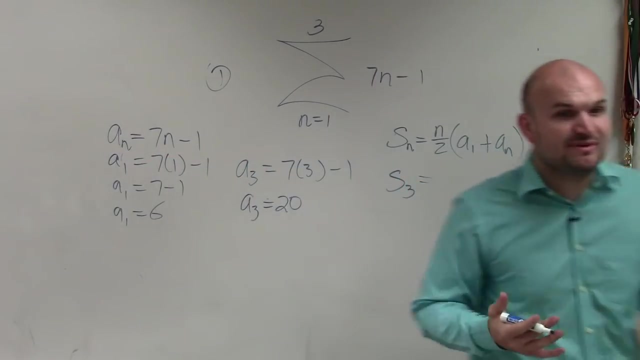 either. All right, I thought you guys would try Mario. still not trying. So now we have s of 3.. We look at this. We say: all right, well, how many terms are we solving? We have starting with 1,. 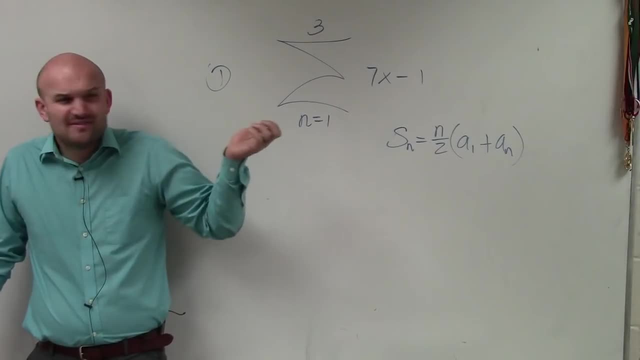 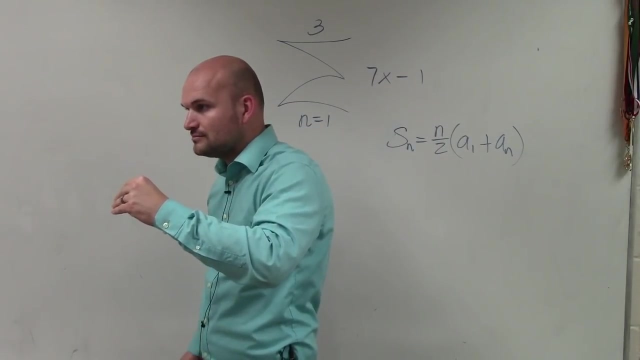 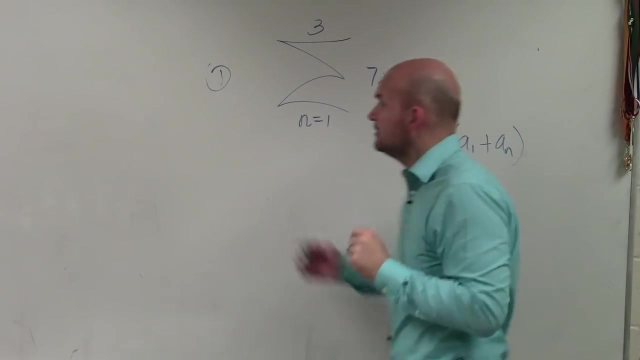 first number is of our sequence. Do we even have a sequence? Well, we only have a formula, this explicit formula, And, if you guys remember, 3, which represents the end. Okay, so if you guys remember how we wrote explicit formulas, 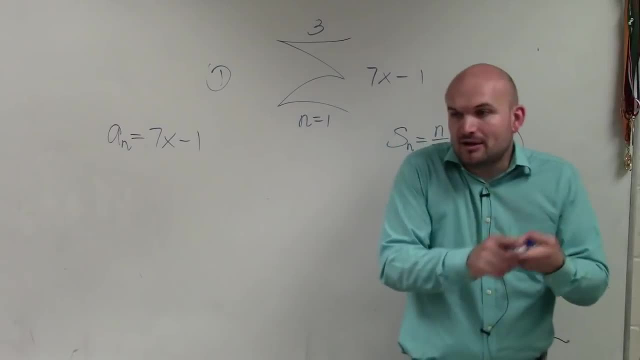 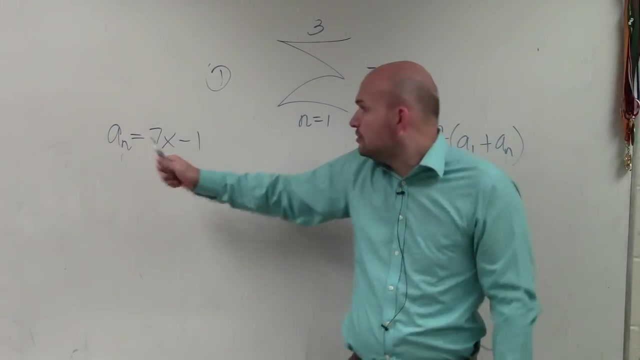 We wrote explicit formulas as like a sub n. right, It could have been arithmetic, It could have been geometric, It doesn't really matter. This is like. your explicit formula can also be written as this: Oops, where n? Where is this x I'm using? sorry? Sorry, there's no x We're using. 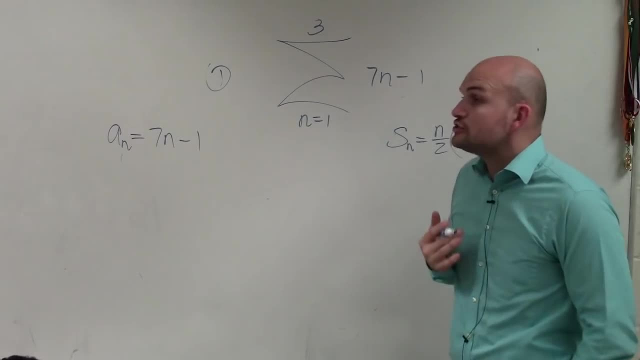 n's here. n represents the number of the sequence. Sorry, I got mistaken. So can we figure out what the first term is? though, once we know what the formula is, Yeah, you just plug in the first number, right. 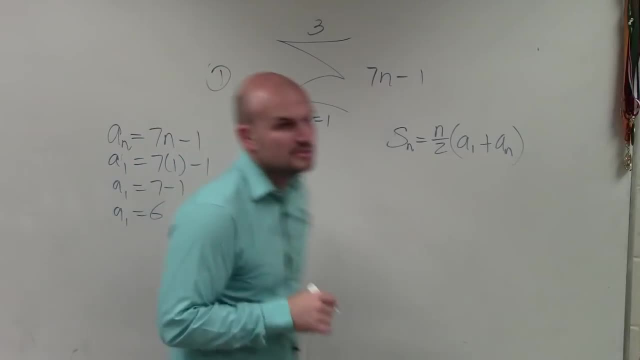 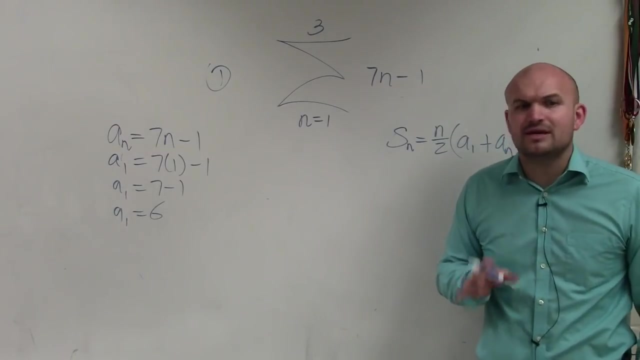 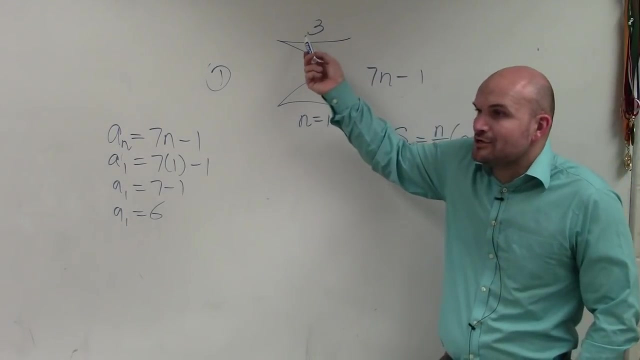 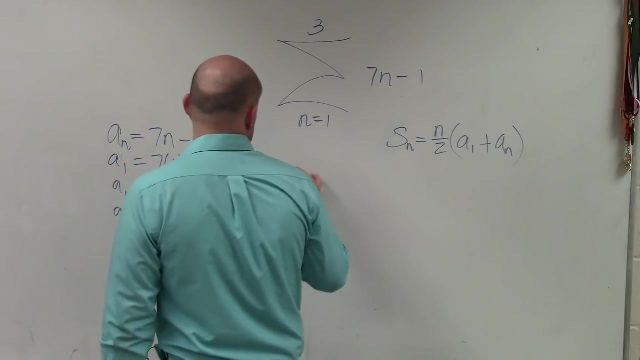 Does everybody see that? Does everybody see that? Okay, now the next thing. Mario, I'm really having a hard time. I really am. The next thing is: what is our last term? The last term is well, what is the last term? it ends with 3.. Can we find out what a sub 3 is? Okay, Yep, So now you just 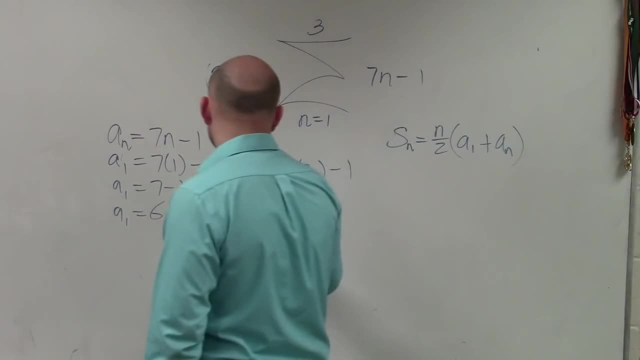 plug 3 in for n 7 times 3 is 20.. So now you just plug 3 in for n 7 times 3 is 20.. So now you just plug 3 in for n 7 times 3 is 20.. So now you just plug 3 in for n 7 times 3 is 21.. Minus 1 is 20.. So Kelsey, 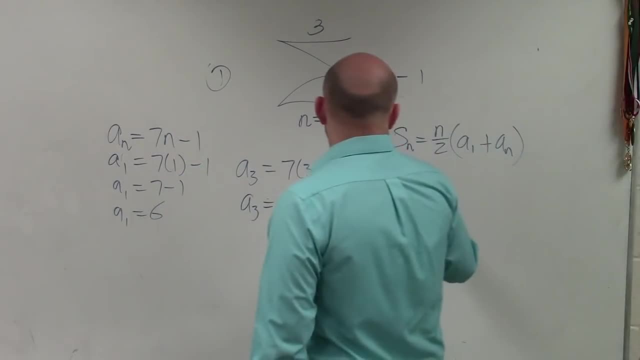 you're not giving it a shot either. All right, I thought you guys would try Mario. still not trying. So now we have s of 3. We look at this. We say all right, well, how many terms are we? 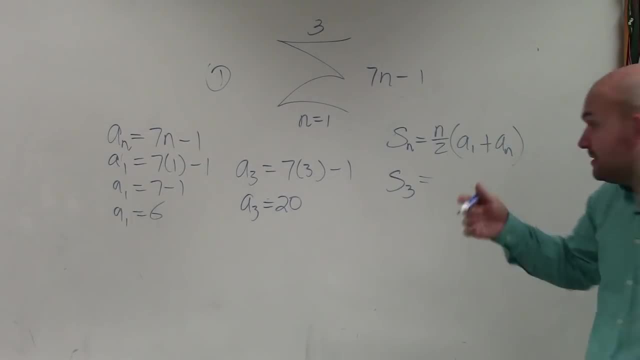 solving. We have starting with 1,, we're ending at 3.. So we are doing three terms. Do we know what a sub 1 is? 6. Do we know what a sub 3 is, Which is because we're trying to find the sum of 3.. So this is: 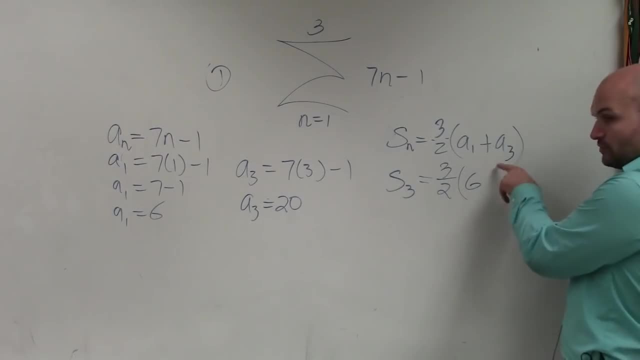 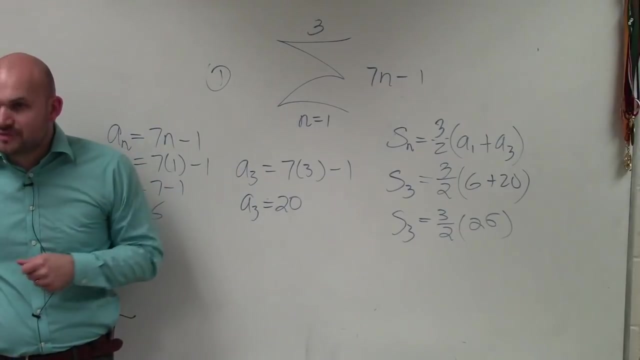 really 3, and that's 3.. So we're really trying to do a sub n which is a sub 3.. So a sub 3, we know, is 20.. So therefore, s of 3 is equal to 3 halves times 26.. How do you multiply a fraction times a?